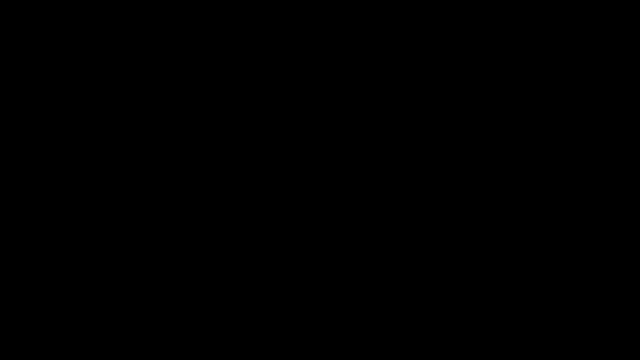 In this video we're going to talk about the harmonic series and if it's convergent or divergent. So consider the series which starts from 1 and goes to infinity of the sequence 1 over n. So if we list out the terms, when n is 1, it's just going to be 1.. 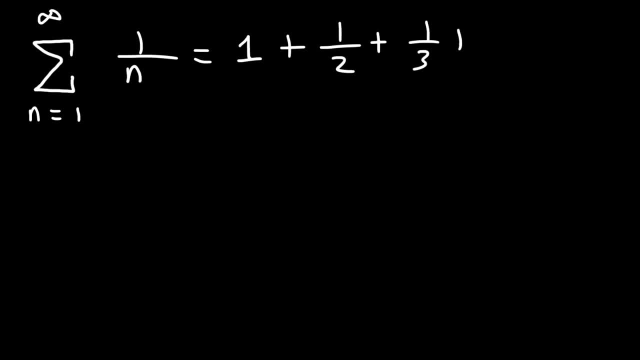 When n is 2, it's 1 half, and then plus a third, plus a fourth, and plus 1 fifth, and so forth. Now, if you keep adding these terms, you'll realize that the sum will continue to increase. 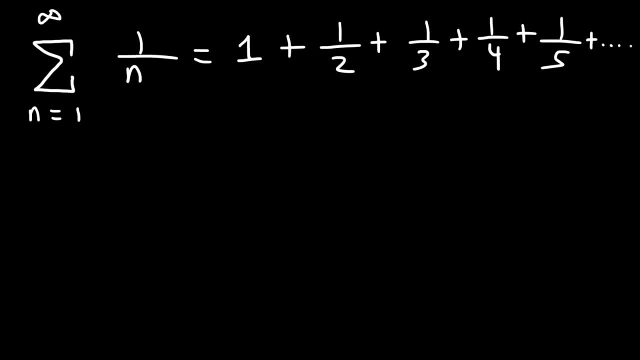 It's going to get bigger and bigger and bigger and bigger. It's not going to converge to a single value if you just add it, And so just by doing that, it tells you that this series is divergent. 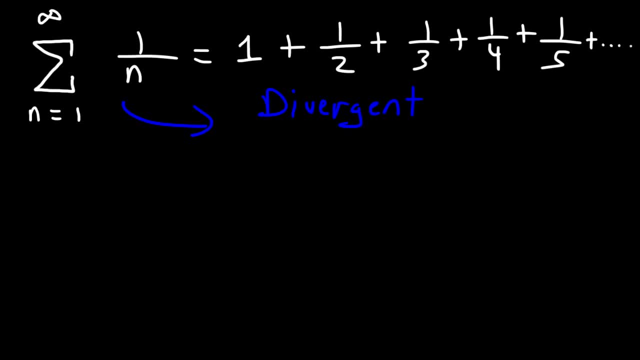 Now, if you're thinking about doing the divergence test to prove that it's divergent, it's not going to converge to a single value. It's not really going to work out too well. So if we take the limit as n approaches infinity for a sub n, so a sub n is 1 over n. 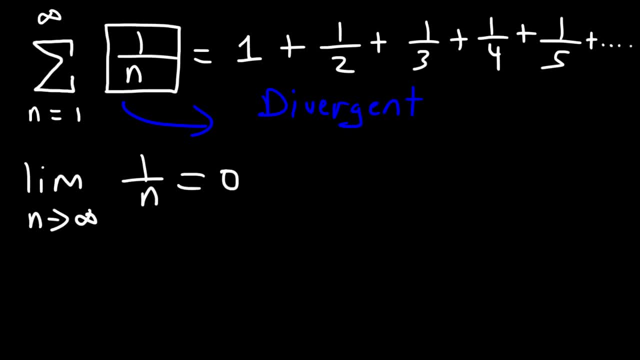 this will equal 0.. Now for the divergence test to work. if it doesn't equal 0,- the limit- then the series diverges. But if it equals 0, well, it's inconclusive The series. it may converge or it may diverge. 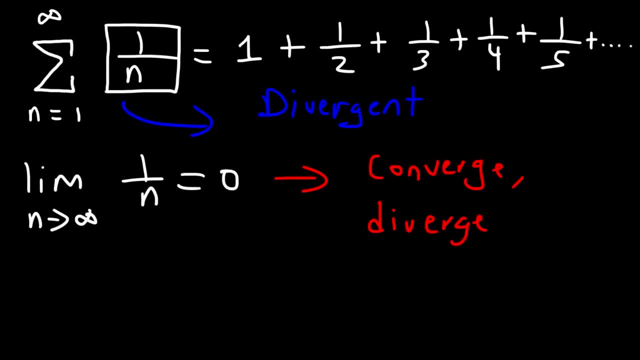 So the divergence test won't help us for this example, But another test that we could use is the integral test. Now, if we take the integral, let's say, from 1 to infinity, of f, of x, dx, if this integral is convergent, then the series, the corresponding series, is also convergent. 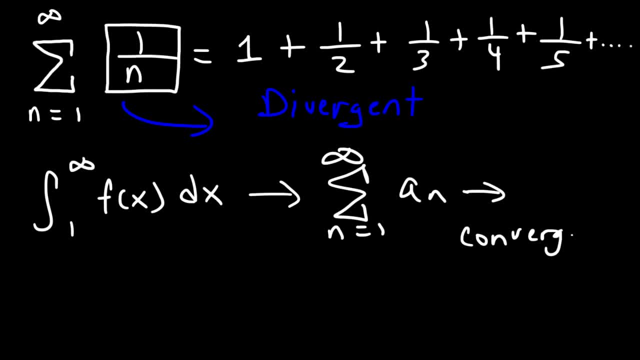 Likewise, if the integral test fails, if it's divergent, then the series will be divergent. So the corresponding function for f of x is going to be 1 over x. So let's integrate it from 1 to infinity.